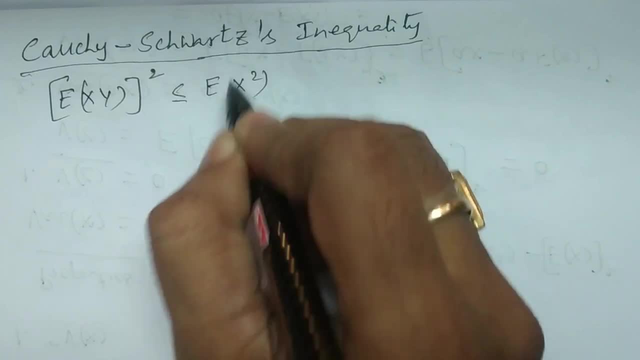 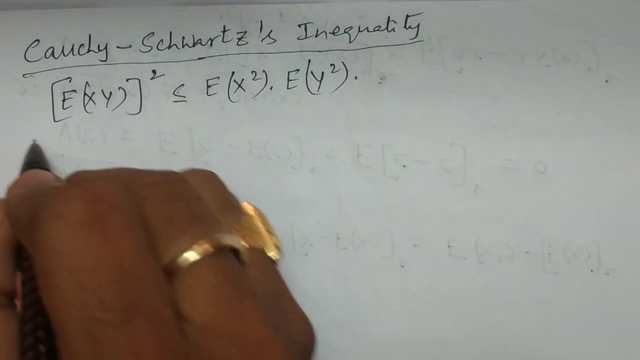 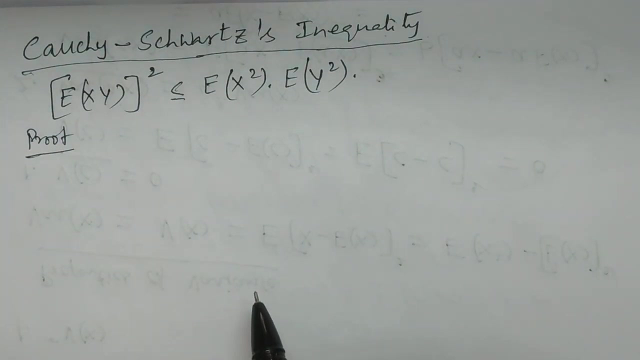 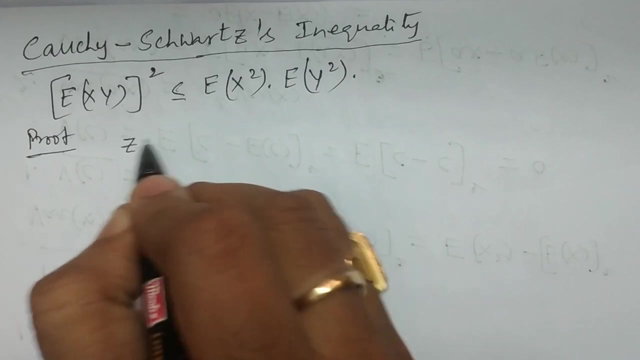 is less than or equal to expectation of x square into expectation of y square. Right? How to prove this? The proof of this particular result: inequality, For which let us consider a real valued function on t, which means which is going to be defined. 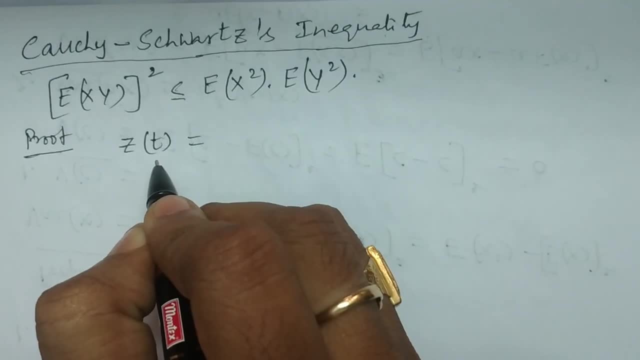 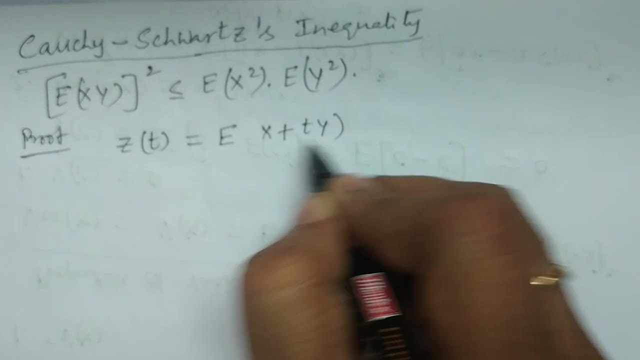 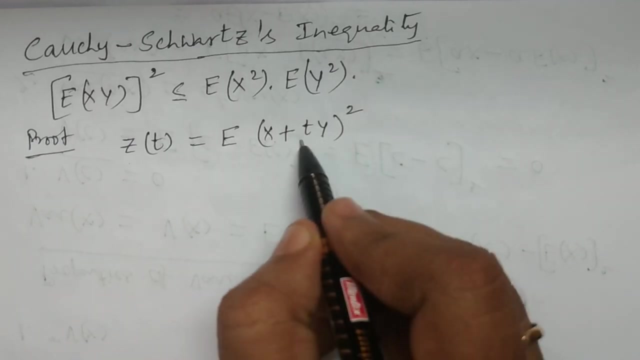 as z of t is equal to. it is a real valued function And it is going to be defined as expectation of x plus ty, whole square. You know for which, if you consider for all the values of x, y and t, this function x. 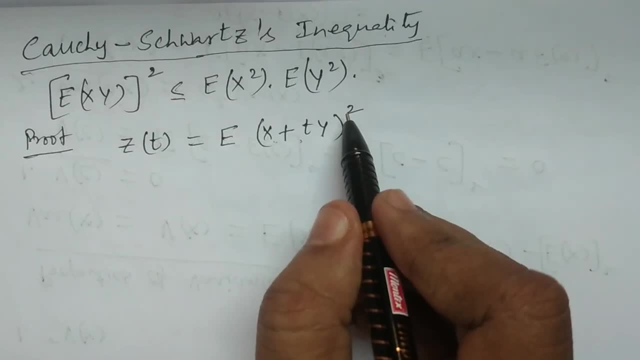 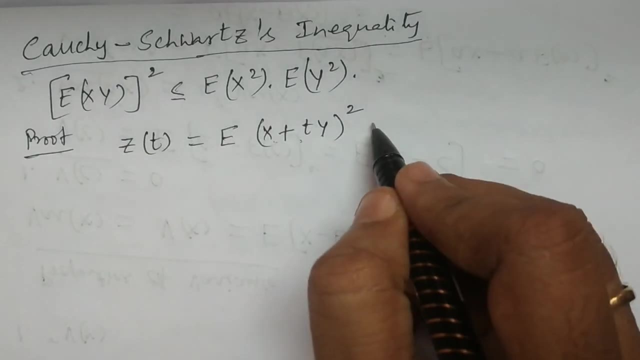 square x plus ty, whole square, which is positive, greater than or equal to 0. So it is expectation. It is also greater than or equal to 0. So therefore, z of t is greater than or equal to 0.. 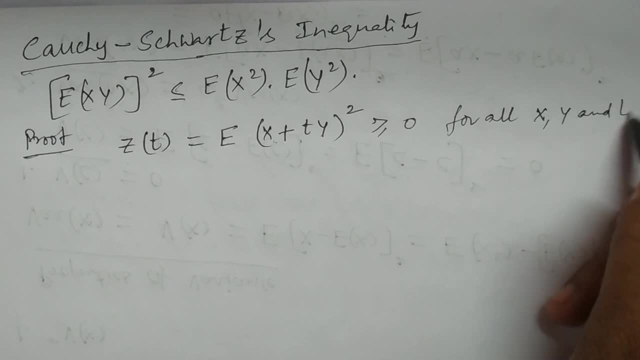 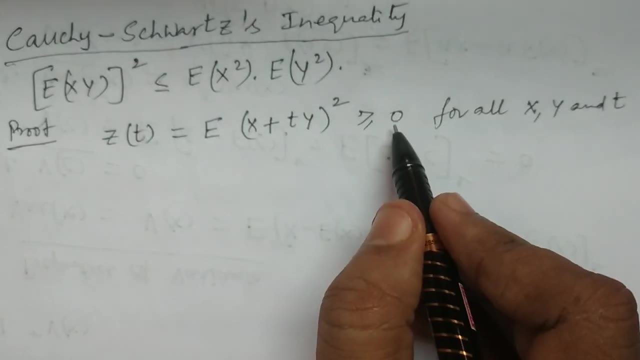 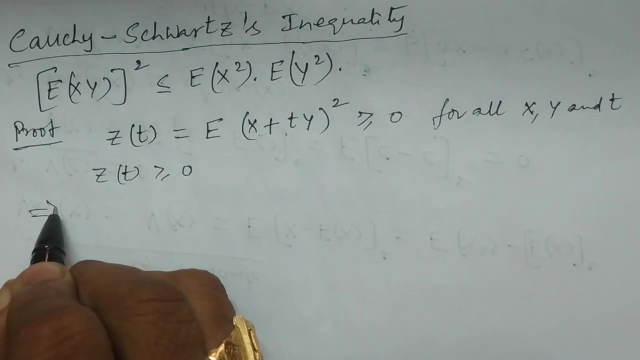 So this is xy and t. For all xy and t, we can have that z of t is always greater than or equal to 0. So which means z of t is if z of t is greater than or equal to 0,, which implies expectation. 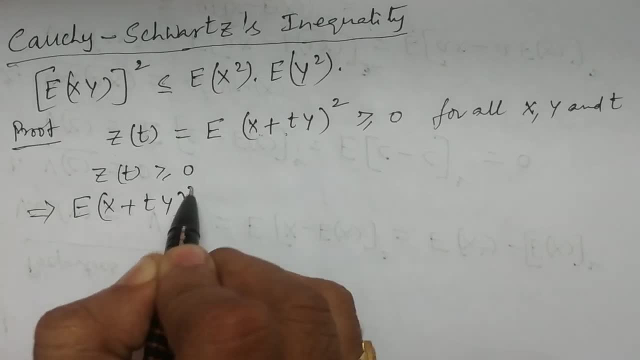 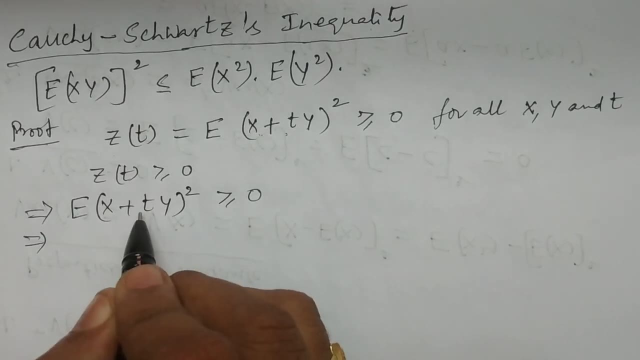 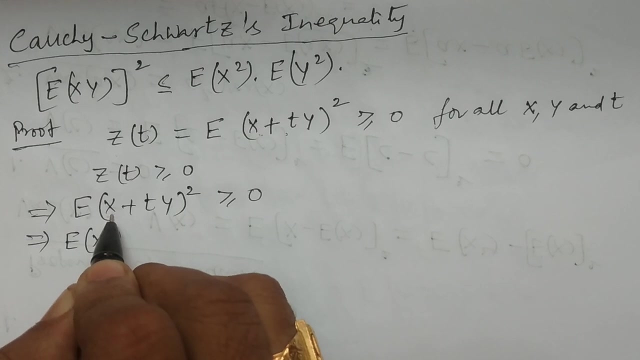 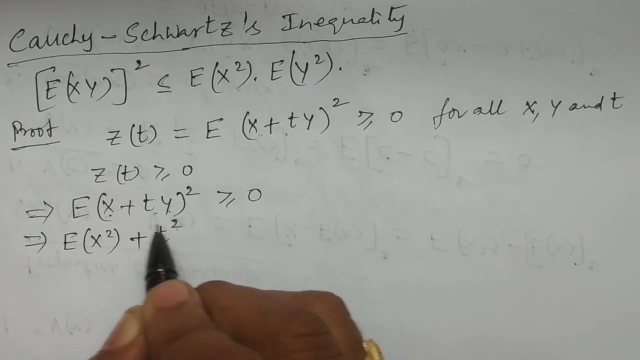 of x plus ty whole square, which is always greater than or equal to 0, which means right consideration of x plus ty whole square. i do square and take the expectations, which means expectation of x square first, first term: a square, x square plus expectation of t square, y square, t square is a, not a value or not a function which 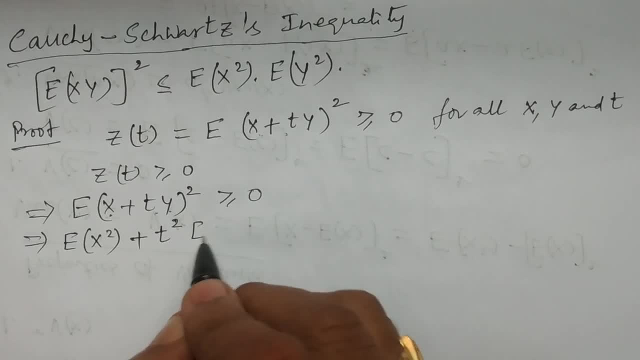 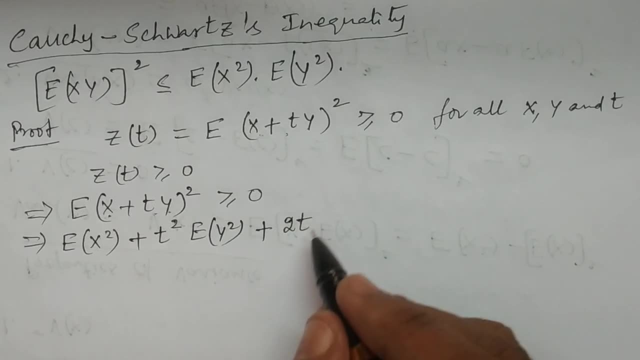 depends on expectation. so t square into expectation of y, square plus 2ab, that is 2 into t. into 2t I am taking outside because of expectations. expectation of constant into x is equal to a. into the constant, into expectation of x. so 2t into expectation of x, y which is greater than or equal. 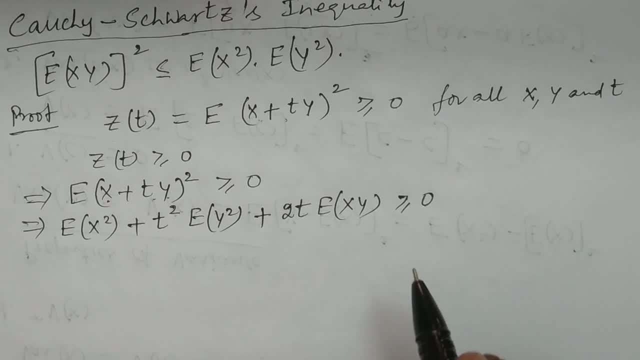 to 0. if you consider this is one kind of quadratic expression in t. so t square, some coefficient, t coefficient and a constant. if you consider t, you consider t, it is a some particular quadratic expression. for example, if you consider t, it is a particular quadratic expression, for example, if 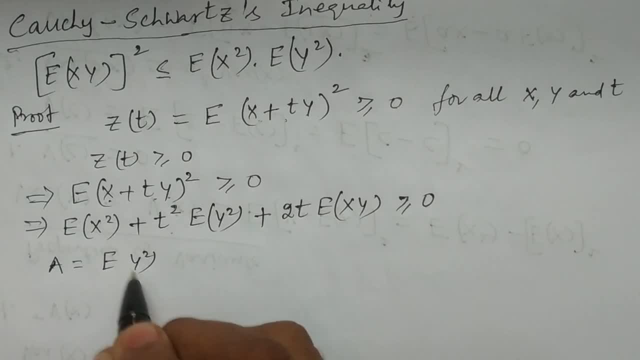 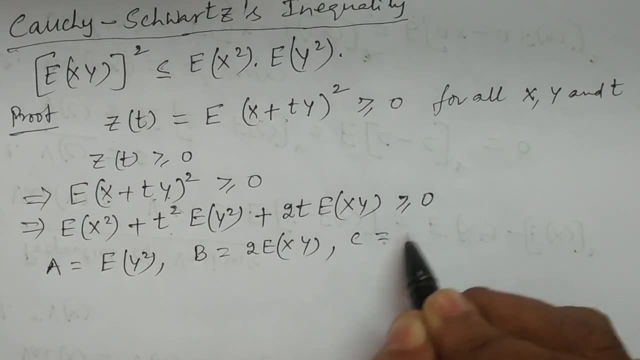 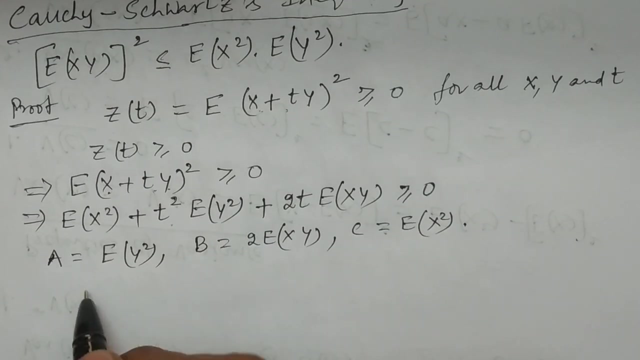 write: a is equal to expectation of y square and b is equal to 2 into expectation of x, y and c is equal to expectation of x square, then it is a quadratic expression in t. if you consider a, t square plus b, t plus c, it is greater than or equal to 0.. 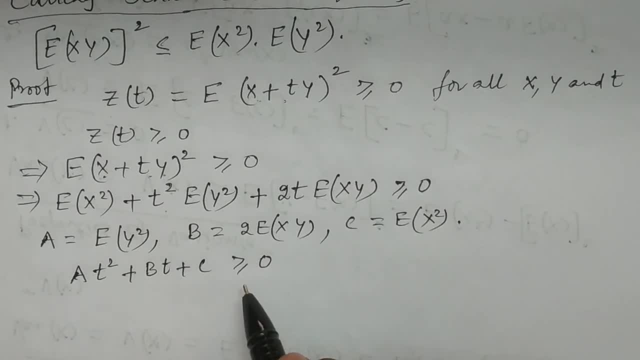 why i am calling as quadratic expression, because it is not equal to 0, it is greater than or equal to 0.. so therefore, this is one such quadratic expression in t, where a is equal to this expectation of y square b is equal to 2, into expectation of x, y, c is equal to expectation. 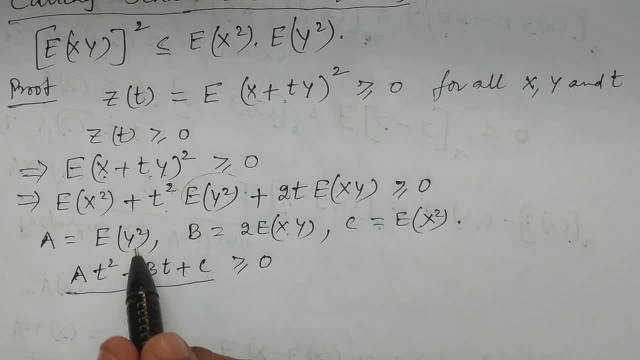 of x square, then this is expectation of y square, a, a, t square, then 2 into expectation of x, y. it is b, b, t plus c. c is expectation of x square, which is one quadratic expression in t. so this is a quadratic expression in t. so what would be the roots for this quadratic expression? if you consider this is a quadratic? 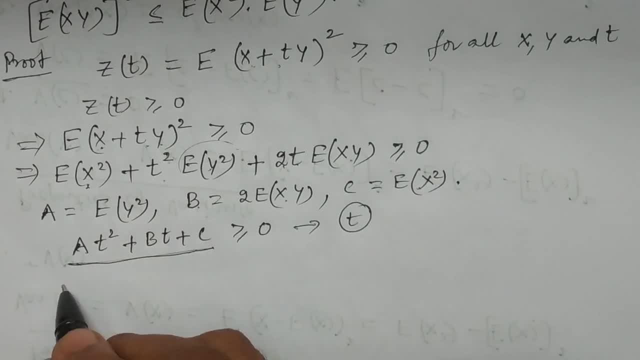 expression, then the discriminant will be b square minus 4 a, c, which will be less than or equal to 0. for this kind of quadratic expression, a? t square plus b, t plus c is greater than or equal to 0. if it is greater than or equal to, 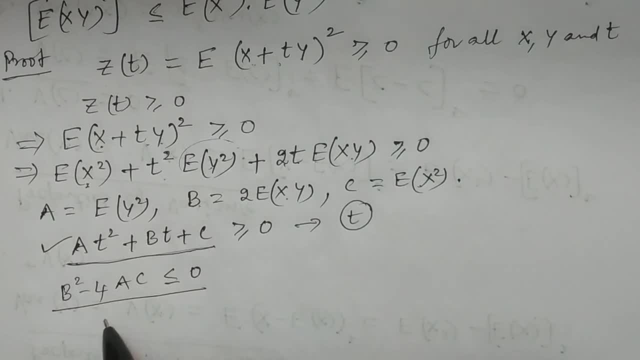 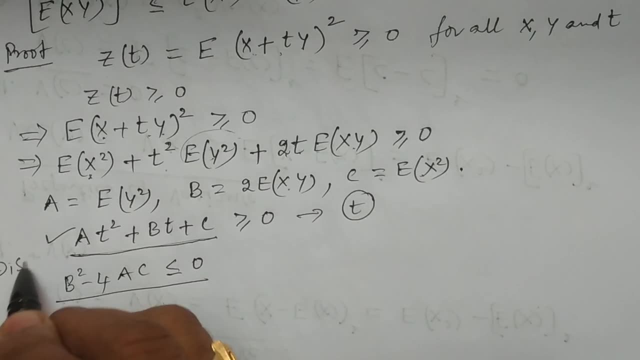 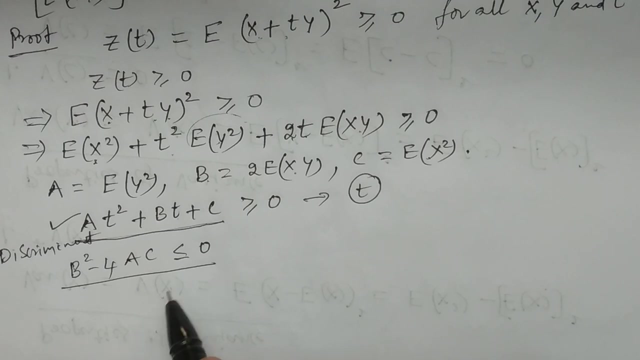 5, then it discriminates: b square minus 4 a. c is less than or equal to 0. then the discriminant will be b square minus 4 a. c less than or equal to 0. so we are considering discriminant. the discriminant will be b square minus 4ac. it is less than or equal to 0. so which means? 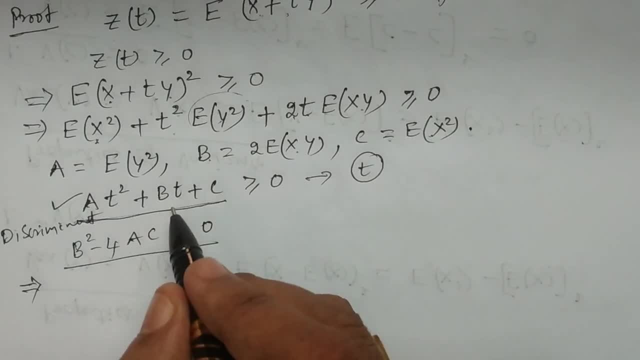 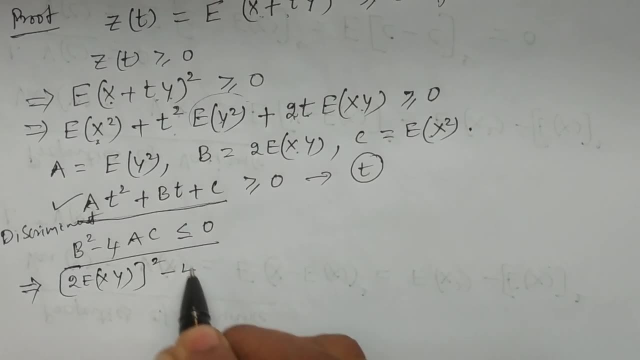 now you substitute the value that b square, that is, b is 2, into expectation of x, y, the whole square minus 4. a. a is expectation of y square and c is expectation of x square. it is less than or equal to 0, 2 square here 4.